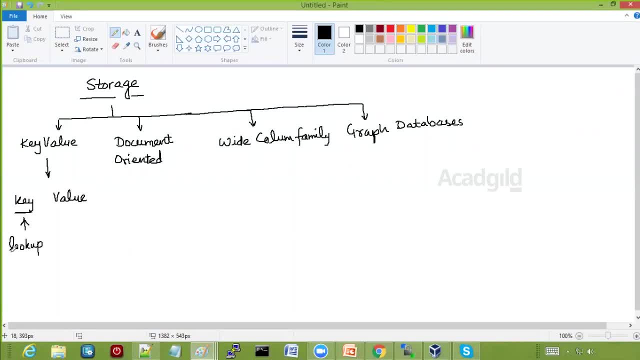 you can compare the key to be the primary key of RDBMS. So there is a key and it has got some value associated with it. Key can be anything: It could be integer, string, any key which is supported, anything which can be converted into bytes And value can contain different fields. 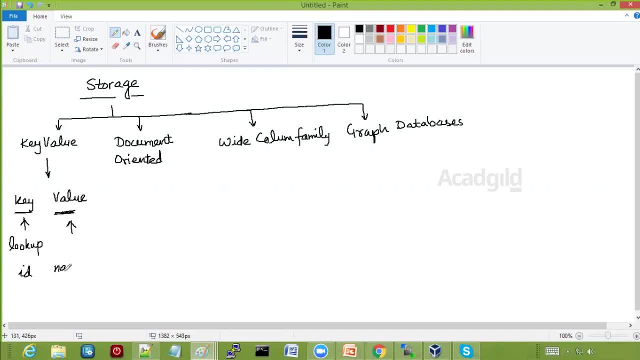 For example, you can have ID as the key and you can have name and age as the value. So these can be the value and this is the key It is. it can be possible in this way, So the lookup on the basis of key becomes very, very fast If you have to search. 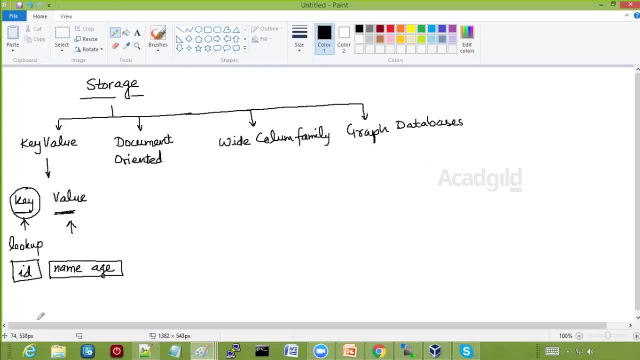 for a particular key and obtain the corresponding value: insertion, deletion, updation or any other activity you might want to perform. it is very, very fast In document oriented database and the example of key value database is HBase. There is a key and there is a value. 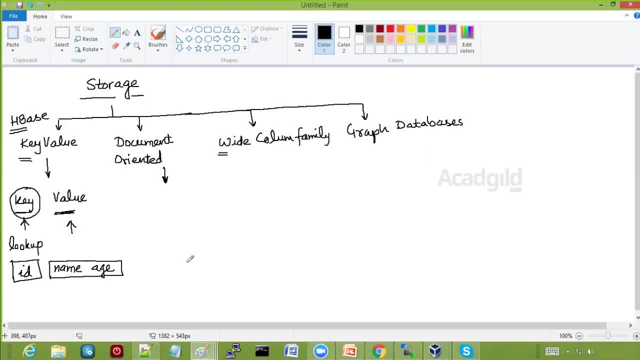 HBase is key value type and it is also wide column family type. So what happens in wide column family type is all columns are collected together in a column family. So you collect columns together in a column family And all the data of a column family is stored together, So you can. 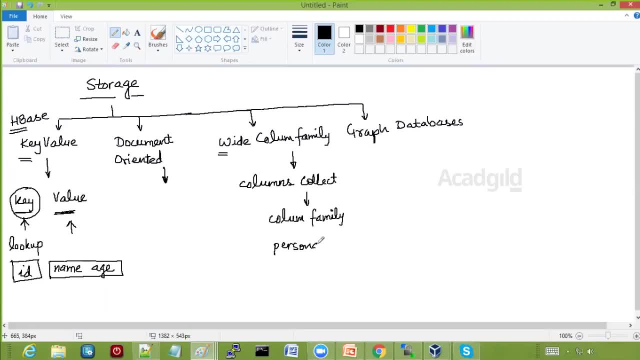 have a column family, say personal details, and you can have a column family as professional details. So inside these are the columns, So they will contain lots of columns. inside that A personal column family may contain fields like name, it can contain like location, it can contain age. So all the columns which are used together. 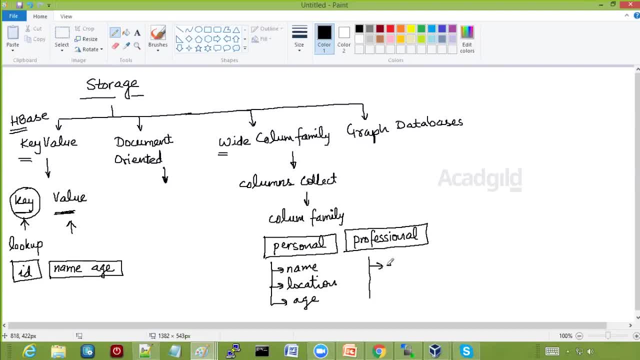 they are stored together in a column family, And professional column family may contain experience, it may contain visa details, it may contain a skill set of the employee. So these things can be considered As a professional detail of an employee And you can have a key as well. So key can be the employee. 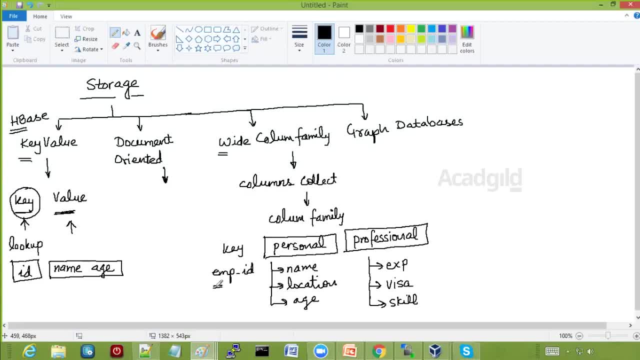 ID, because every employee is having a different employee ID. So HBase is both: HBase is key value type and it is wide column family type database as well. So again, this is like how data is stored. The classification goes on that level If we talk about document oriented database. 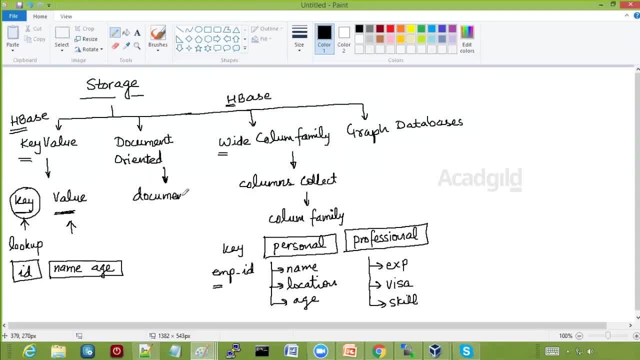 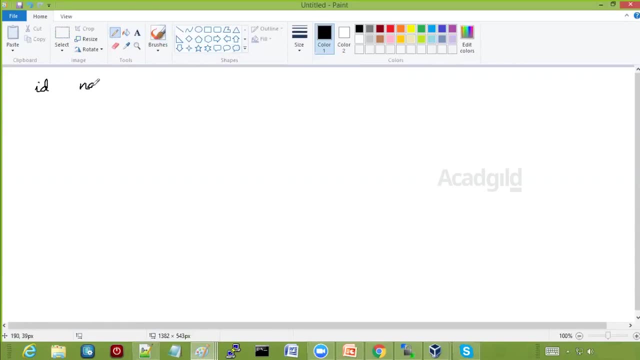 they contain documents And one document is like one, one column of sorry, one record of an RDBMS. To give you an idea, if in RDBMS we have got something like this: there is ID, there is a name, there is age, for example. So ID is one, name is, A age is. 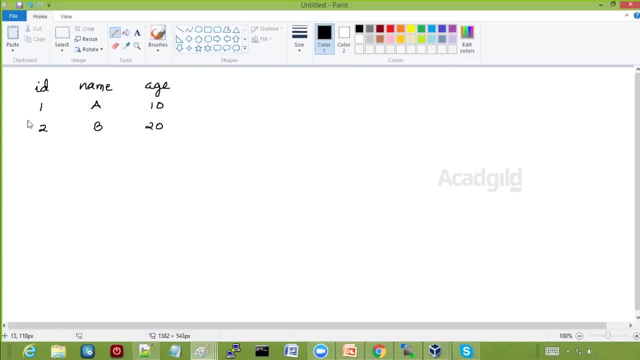 10,. ID is two. name is B, age is 20.. So there are two records In document oriented database. they will be stored as a document, like ID it is one, name is A, age is 20.. So there are two records. 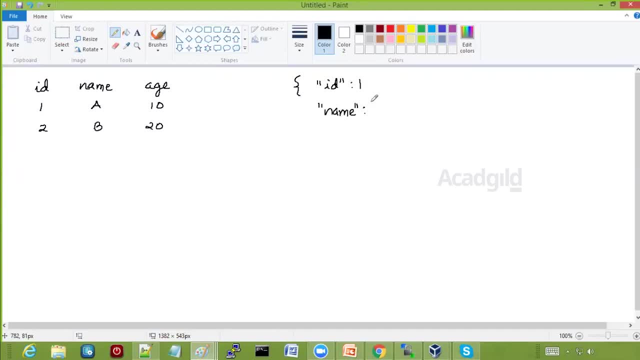 One name. name is a string, So it can be A age, So age can be 10.. So this is one document, what we call this as a document. So it corresponds to one row of an RDBMS, So 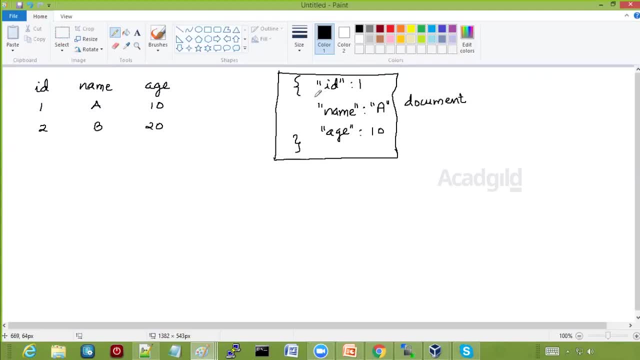 this is a document And a collection of document is a table And you can easily see these are the different fields of the particular document. So these are the fields. Again, they have dynamic behavior And a collection of document is analogous to a table, which is called as collection. So 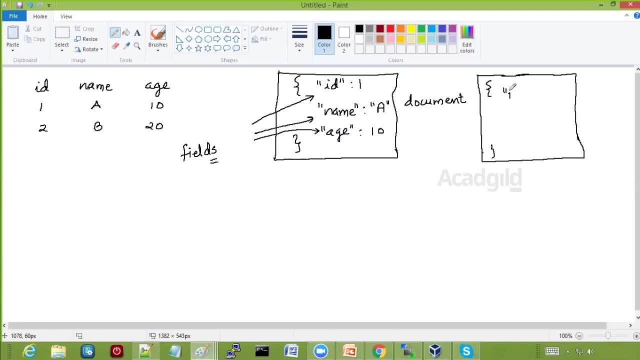 we call them a collection. So different document can have like this: It can have ID as x, y, z. You can see, here the ID is integer, here the ID is a string. So different documents can have different schema. that's perfectly fine And it can have a location as a column or location as a. 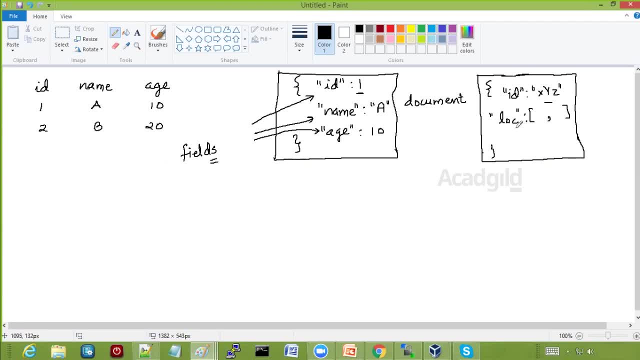 field and location can be an array as well, like in terms of latitude and longitude. So you can see, you can come for all the dependencies like this: For example, if you could have a simulation, you can ask a doc which gives You know. you can go to XML mornings and you would save your 건 erw 시간 to to talk to the data myself. Or you can go to JSON That Union those days you can call a say and you can call objects on excel and View report. 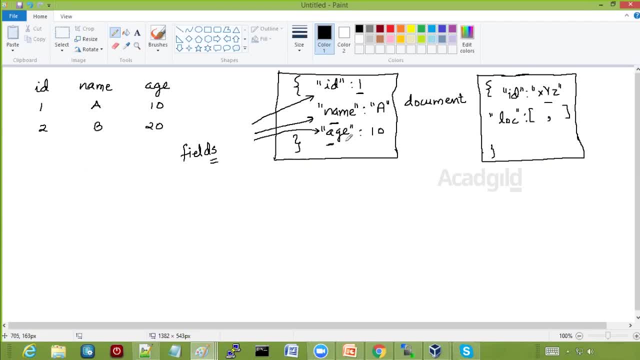 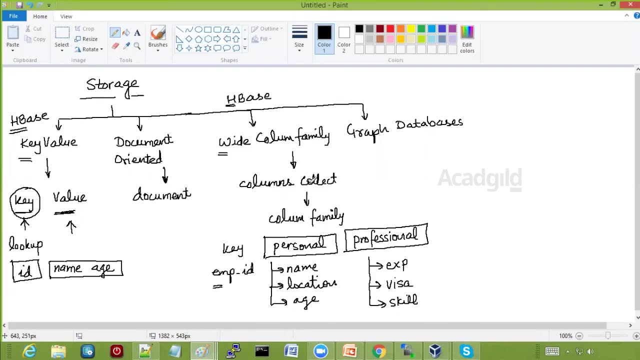 can see, it's completely dynamic. the name and age are not here, so different documents can have this is document one and this is document two, so different documents can have different fields, different types of fields as well. so this is also one type of databases which fall under the. 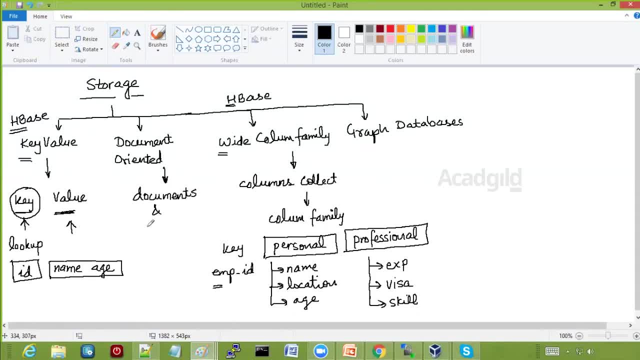 category of document oriented, so they contain documents and collections, and they also contain collections. are like tables, documents are like rows and they also contain databases, so inside a database you can create multiple collections. one example of document based database is mongodb, which is a very popular document based database, document oriented database, and many times we 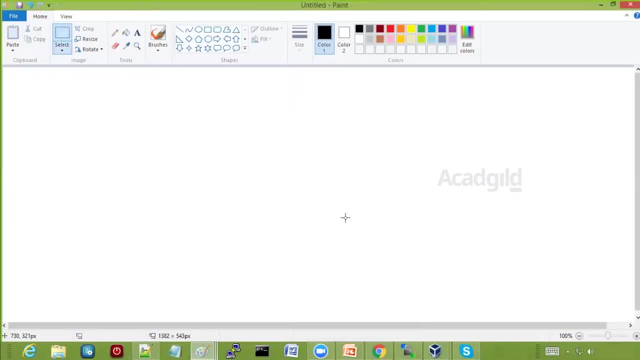 require graph processing. like graph processing may look like: uh suppose, if you talk about any facebook post, so there is a post and there is a user u1 who has created the post, so it creates the post and in the post, two users were tagged. you know, you can tag some persons in the post. in this particular post, the post name is p1. 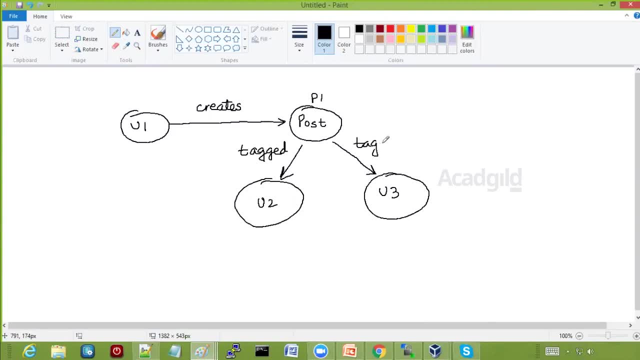 tagged. so these are the two users who have been tagged in the post going forward. there could be, like, say, user u4 who has commented on the post- he comments on the post- and there could be something like their eyes. is some user u5 who likes the post, who? and there could. 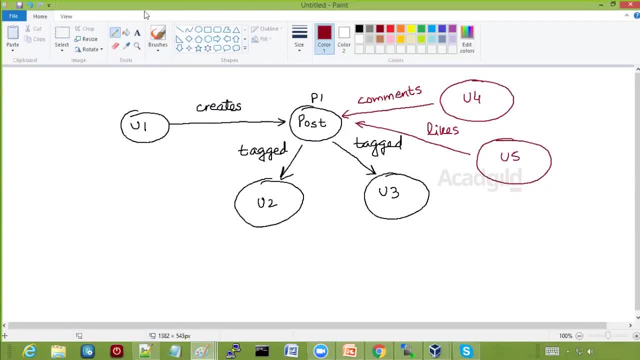 be multiple user who likes the post. so you see, the conclusion is you can have a lot more features. there is lot more relationship in rdbms. these relationships can be represented in the form of different tables, and suppose i want to answer a question. my question is: what are the? 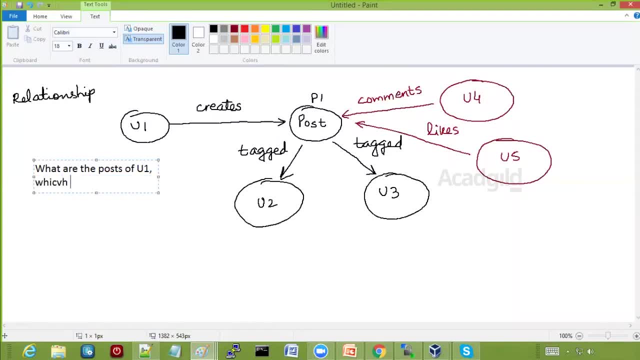 posts of user one which were liked by at least one, at least one user and commented by at least two users. it could be like that, or you can go ahead and add more features and tagged at least kind of three users. so you see, this is our one question which i would like to answer. so if you, 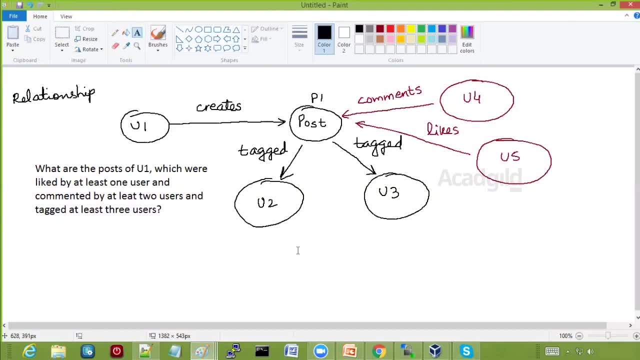 want to answer these kinds of questions. so, since there are lots of relationships, you have to make lots of different joins in the rdbms, because i have to go for the post of u1, which were liked by some, which were commented by some, and then, though those posts, tagged some users in order to have 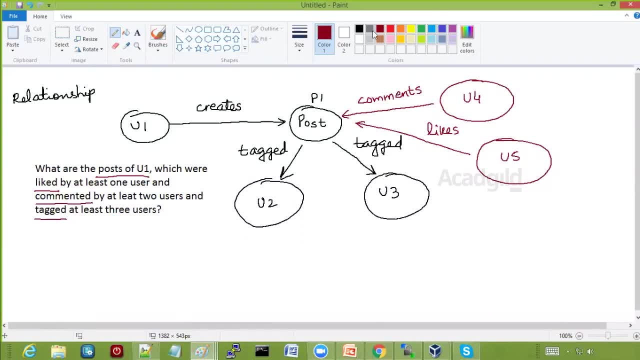 these things in place. uh, let's say i want to make a post of u1, which were liked by some, and those posts tagged some users in order to have these things in place. you create a cảm find which could be a post of us, but that one is what you have to fit and if you